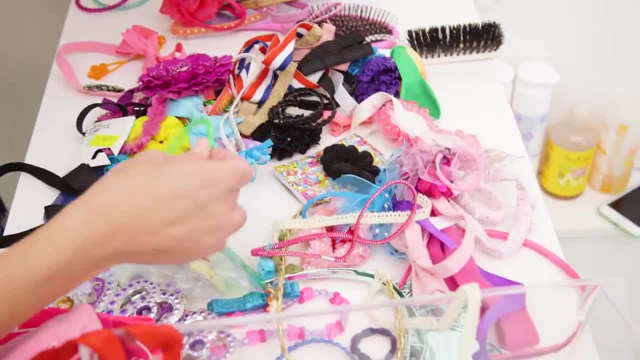 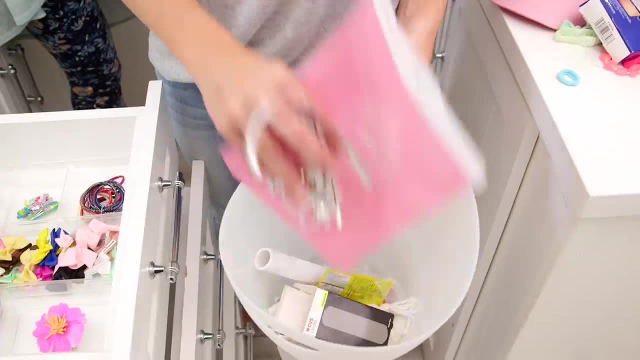 Number three: pile it up into keep, donate or trash. Girls come with so much stuff. Press has a thing with the spiky headband, So we donate all of those And a lot of things were broken. I ended up finding a few things of my own. 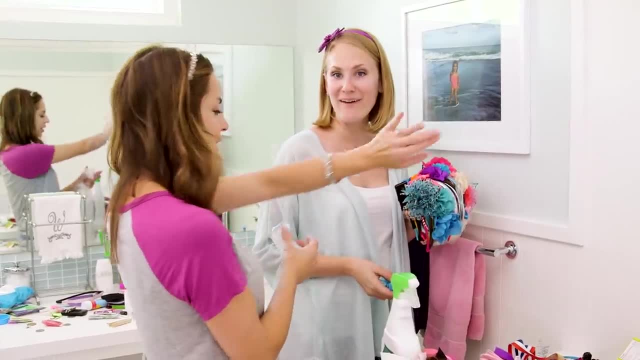 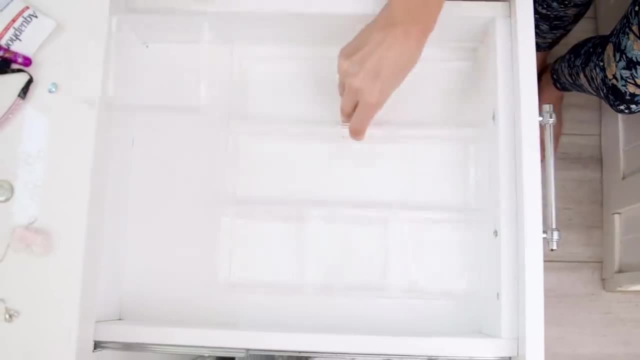 I've been looking for this bracelet. This is so cute. And then, number four: choose containers. Katherine is so good at this. I love these clear ones- Perfect. They slid around a bunch. So we added these blue dots to make them nice and secure. 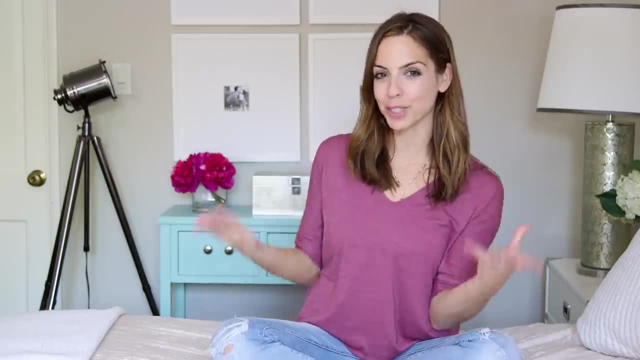 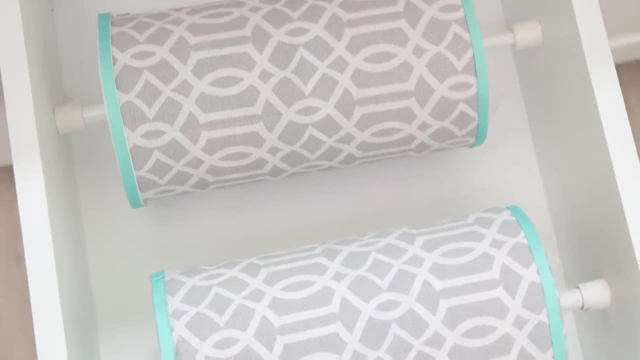 Boom For the headband drawers. Brooke made this beautiful DIY holder using an oatmeal container and pressure rods. She's going to show you how to make it, But just a little sneak peek. How awesome does this look? And then, for under the drawers, we found these tall and thin containers that worked with the plumbing. 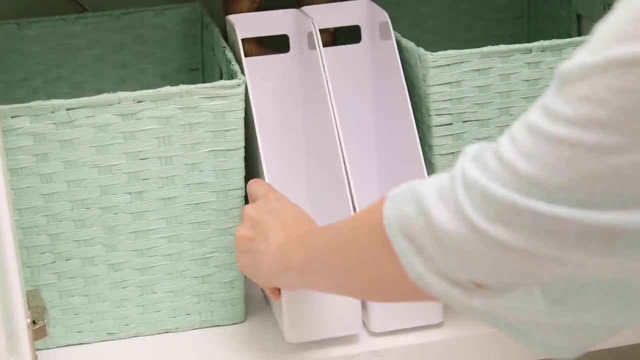 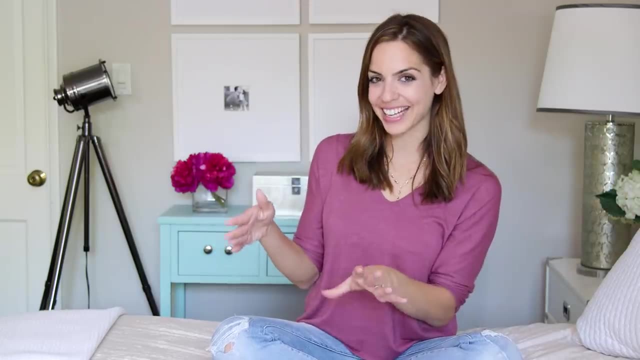 And then Katherine recommended these magazine file holders: So inexpensive and great for little items. Then number five: decant and arrange. So this is putting everything in. Katherine does not like packaging. There's one thing I've learned from you: It's to decant. 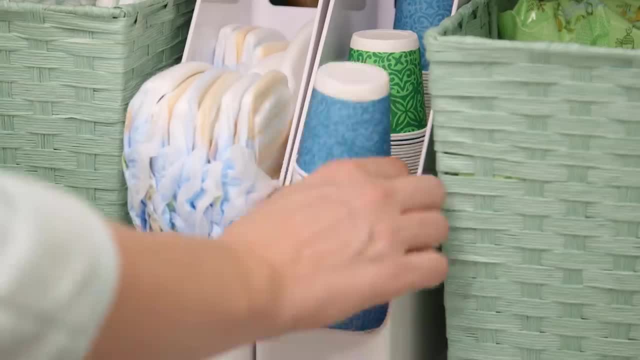 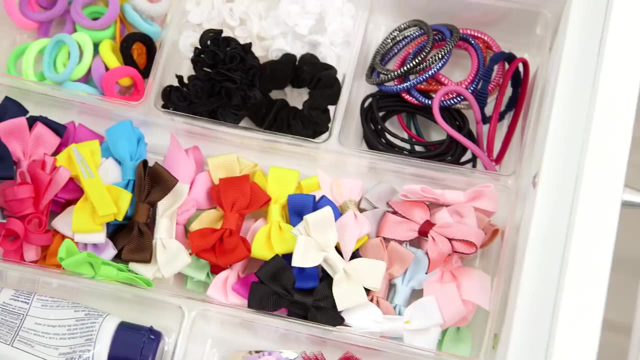 So we had the band-aids and the kids' diapers and all those cups that they use. Unpackage them. It looks amazing. Look at how perfectly it fits a hair dryer. I love that. And then we just made sure that everything like the bows had their place. 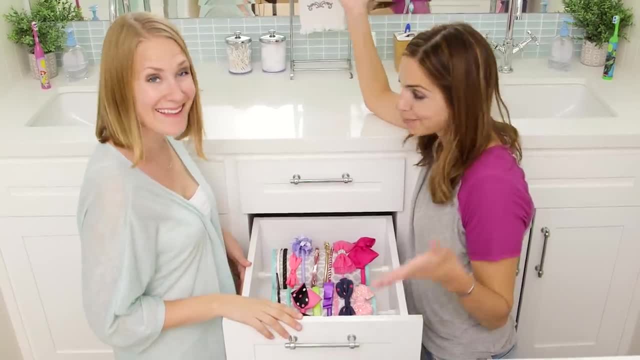 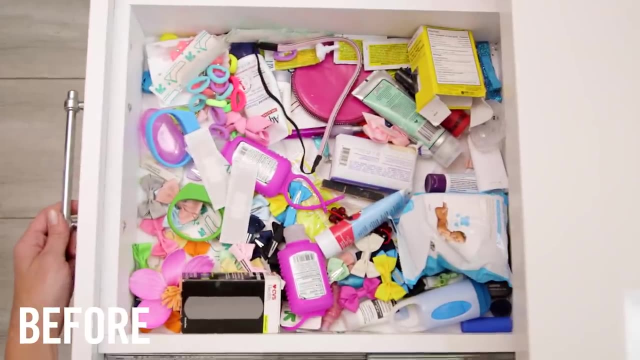 And then, of course, the headbands. Is it weird how happy this makes me. This looks so amazing. I can't wait for Presley to see this. So here it is, guys, The befores and the afters. This is the first and the last. 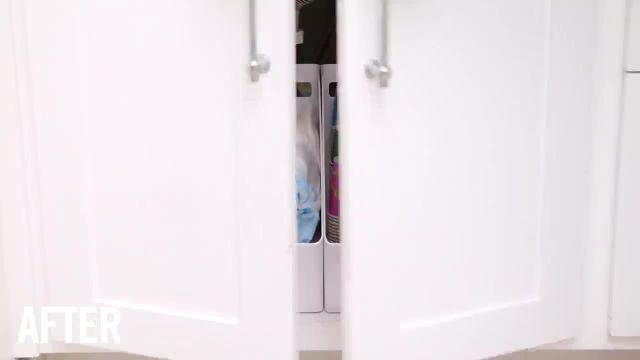 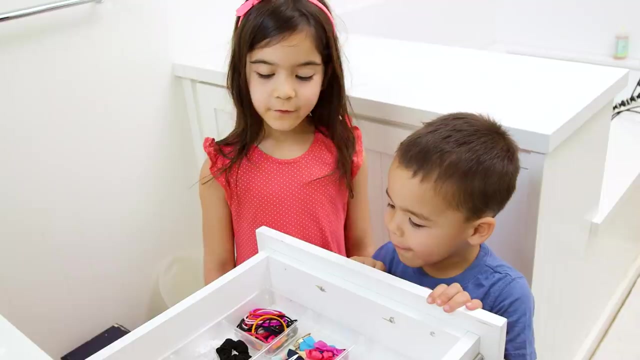 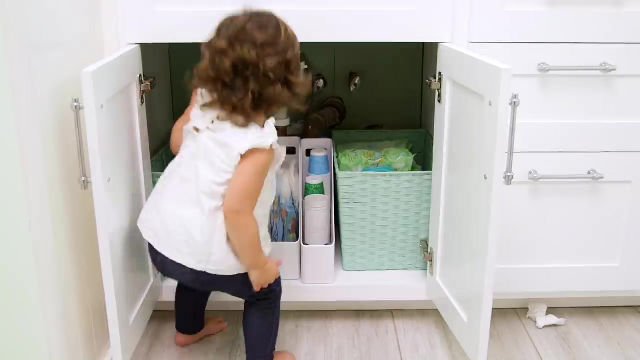 And then the second. Well, here are the firsts. Most importantly, Presley is so happy with it. It helps her get ready in the morning and she is determined to keep it clean. Fourth, we got to keep her organized. Even Tess was impressed with the difference. 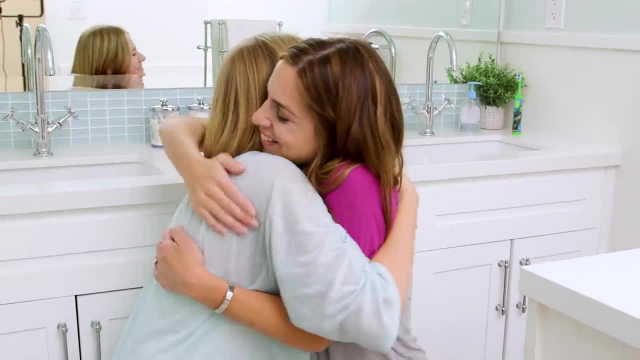 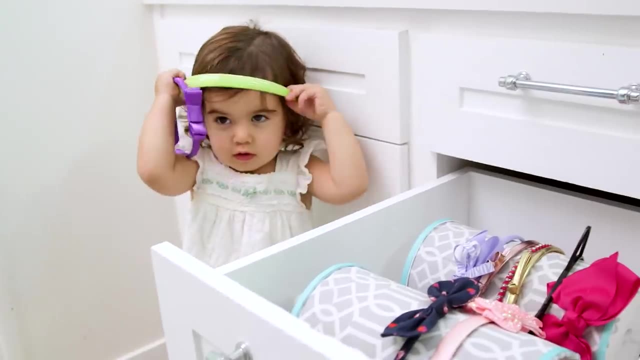 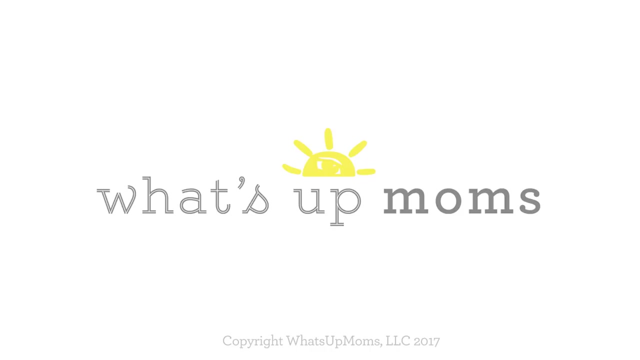 Yay, Thank you. Yeah, Huge thank you to Katherine for yet again turning my space around out her channel. I will see you next week. Bye, We're not going to tell your sister, we're in here.